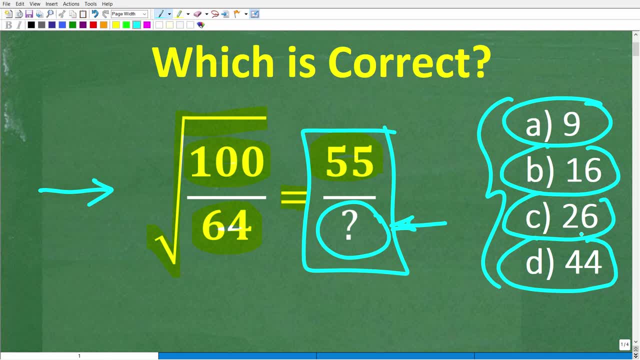 use one if you think that's going to be the difference in terms of you solving this math problem. But if you have the answer, go ahead and put that into the comment section. I'll show you the correct answer in just one second. Then, of course, we'll walk through. 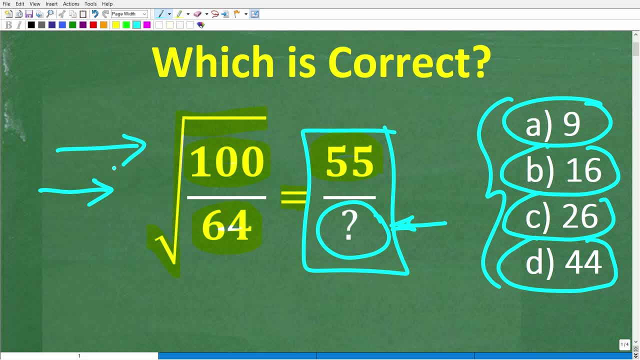 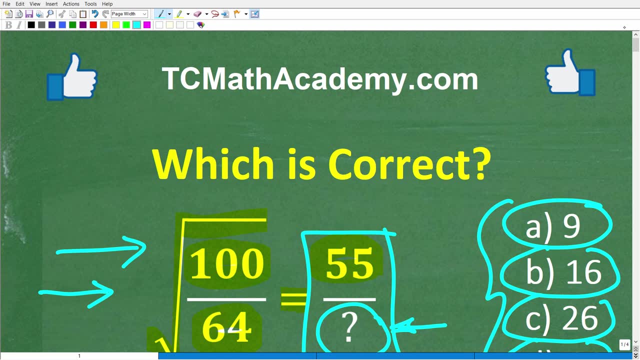 it Step by step how to solve this math problem. But before we get started, let me quickly introduce myself. My name is John and I have been teaching middle and high school math for decades. And if you need help learning math, well, check out my math help program at tcmathacademycom. You can 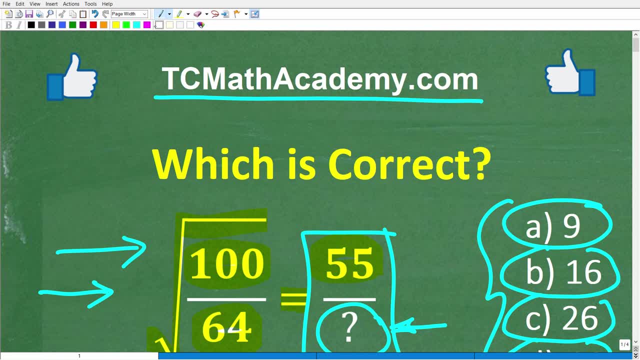 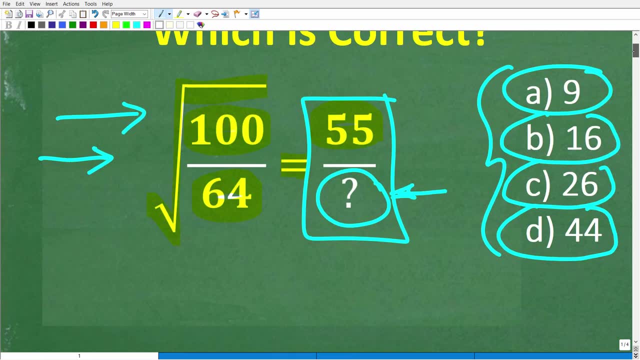 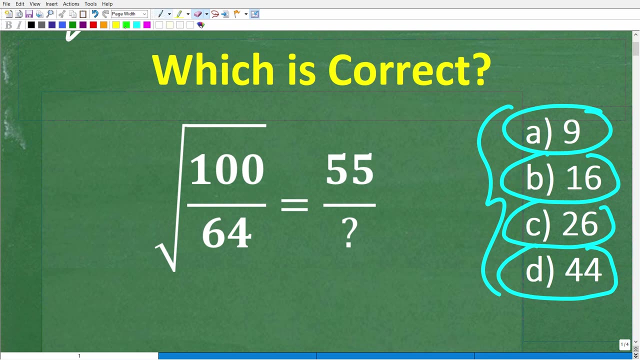 find a link to that in the description below, And if this video helps you out or if you just enjoyed this content, make sure to like and subscribe, as that definitely helps me out. All right, so here again is our problem. And you can use a calculator, but try not to use a calculator. That's the kind. 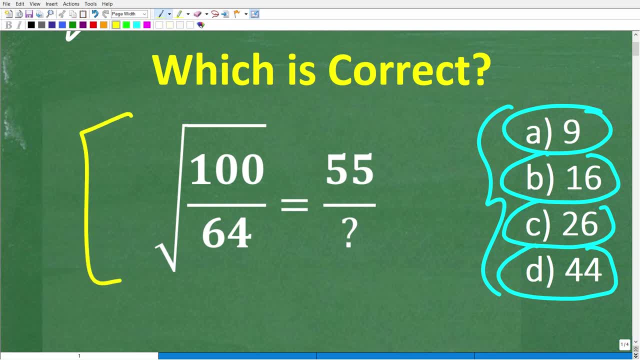 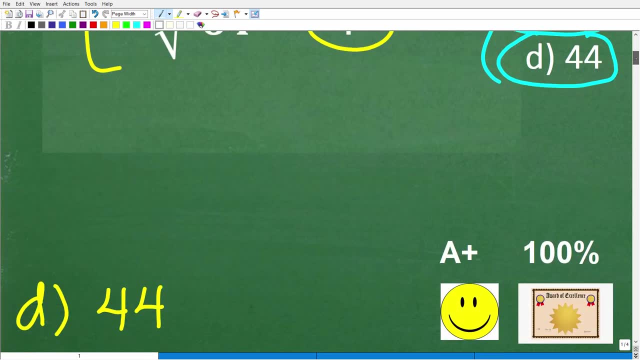 of best way to do these problems. So the square root of 100 over 64 is equal to 55 over what number? Let's take a look at the correct answer. The correct answer here is D 44.. Now, if you got, 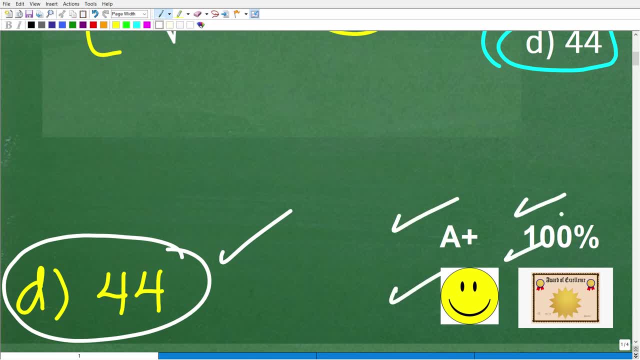 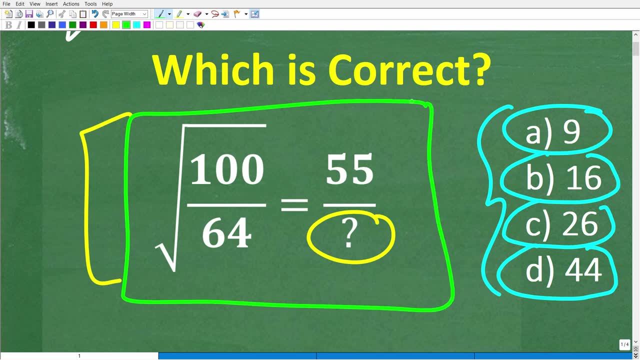 this right, you definitely get a happy face, an A plus a 100% and a certificate of excellence, because you appear to be a certified professional expert in the area of solving a proportion problem. Now, if you don't really know what a proportion is in terms of mathematics, probably most of you have heard that word. 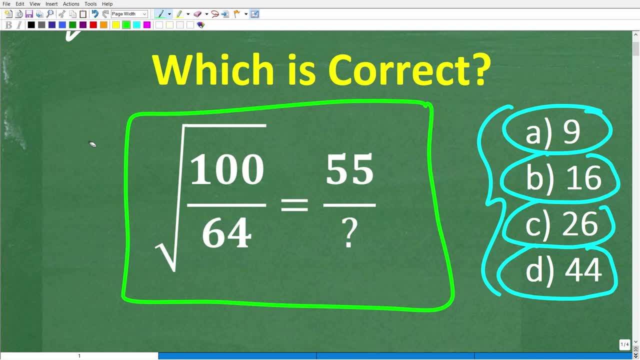 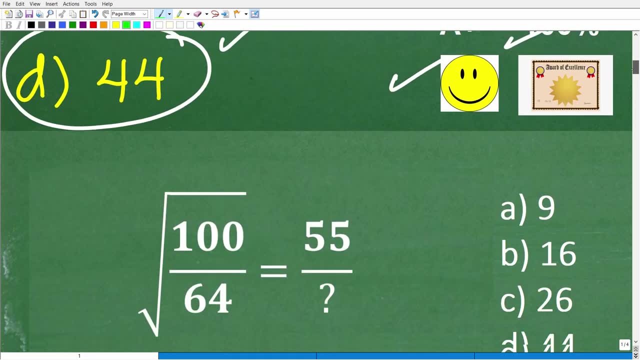 right Proportion: something's in proportion or proportionate to something else. Well, that's what we're talking about, And this is a big deal in math, And it's the concept that I'm going to basically be teaching in this video to solve this problem. Now I'm going to define what. 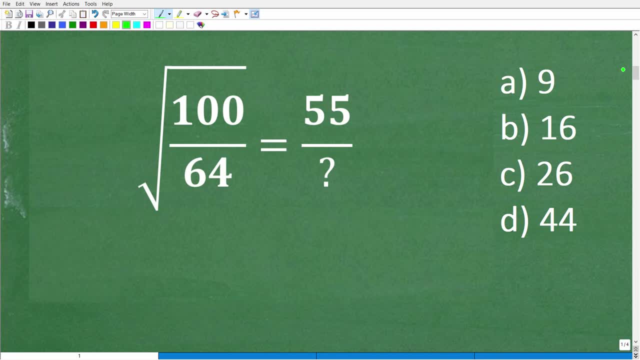 a proportion is here in a second. But let's just kind of take a look at this problem And let's suppose you were facing this on a math test or quiz. What should you do? if you don't really understand the problem You might be. 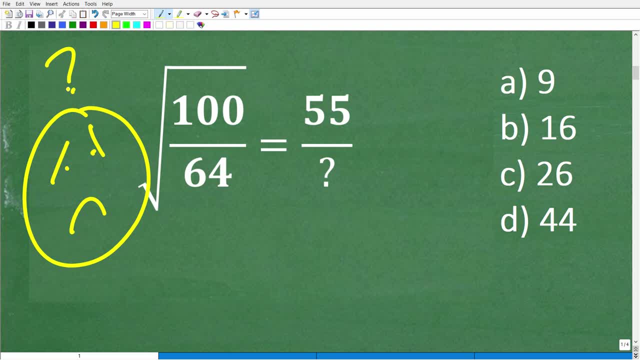 saying: hey, Mr YouTube Math Man, I totally don't even get this. What should I do? Well, you should take a guess, right? You got one out of four chance to get the right answer. So for those of you that, 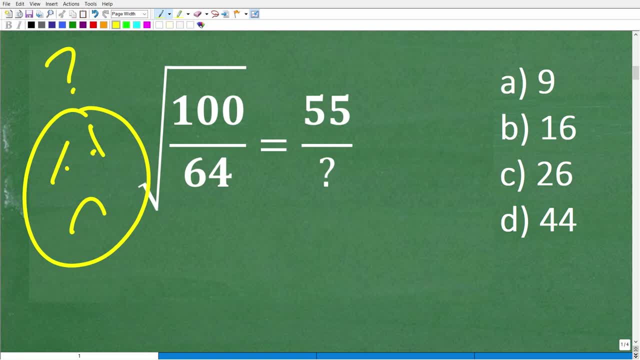 are still math students or still have to take exams. never, ever, leave a question blank right, Especially a multiple choice question blank, Unless you're going to get penalized for a wrong answer, And that could be the case on some tests like the SAT, But in this situation you might be like: I don't know, maybe the answer is nine. 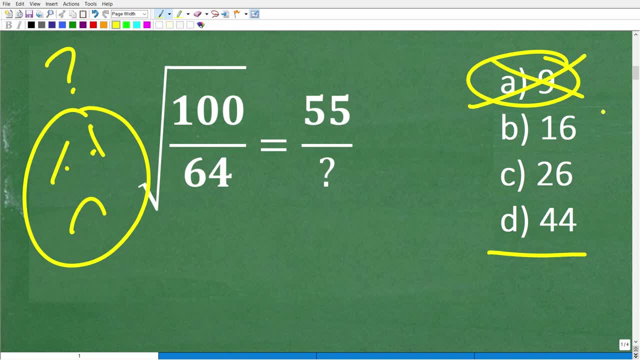 Well, that is a fantastic guess. Unfortunately it is wrong. But what you could do if you were allowed to use your calculator is basically take the square root of 100 over 64. You know, maybe you can kind of get someplace with that. you can get some sort of value over here, But really, 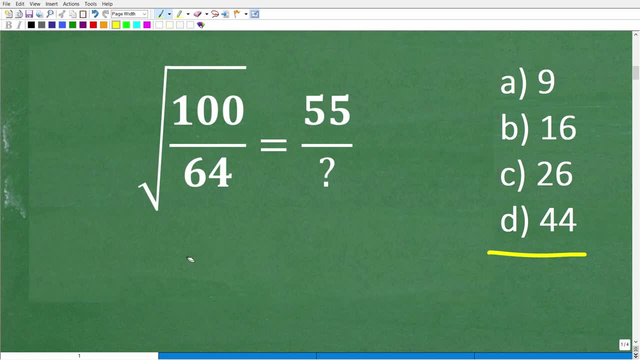 the best approach to solve this particular problem is to just do the math. Now, here again, the answer is D, Okay, meaning that 55 over 44 is the same thing as the square root of 100 over 64.. Now, hopefully some of you could- you know, they're pretty good with fractions- say: well, 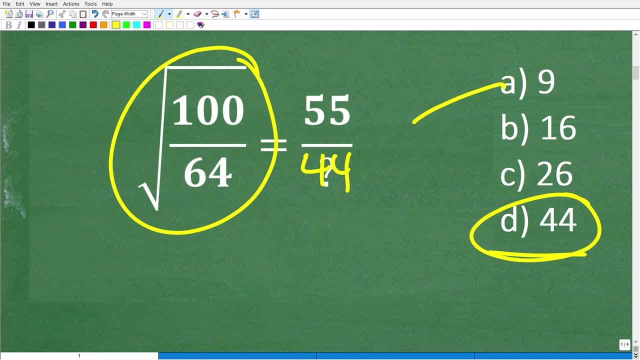 I have the square root of 100 over 64.. You know, you could plug in these various numbers down here in the denominator. you'll see that this fraction is equivalent to this fraction. But let's just go ahead and get into the actual mathematics of it. Again, we're going to be using something called. 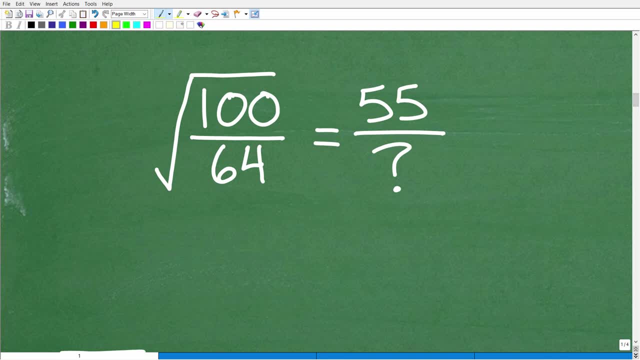 proportions. Okay, now, here is our problem, And there's a couple different things going on here. So we have this square root, square root of 100 over 64. And it's equal to this fraction. So the first thing that we want to address is this square root situation because, hey, maybe we can make 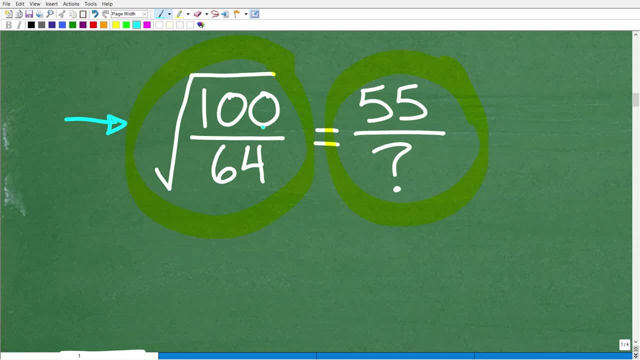 this problem simpler. So we look at this, these numbers in this fraction 164,. you might be saying, Mr YouTube Math Man, I'm really good with square roots. I know that the square root of 100 is 10.. And the square root of 64 is eight. Well, that is good thinking, because we can actually 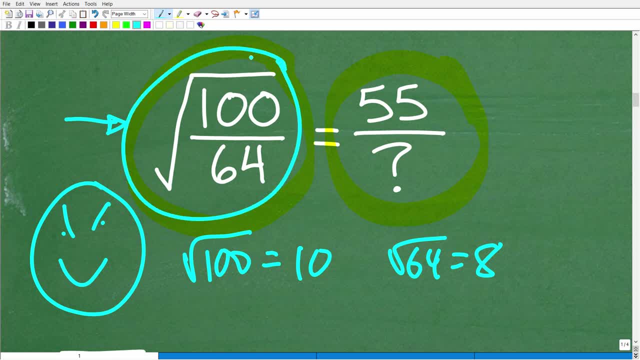 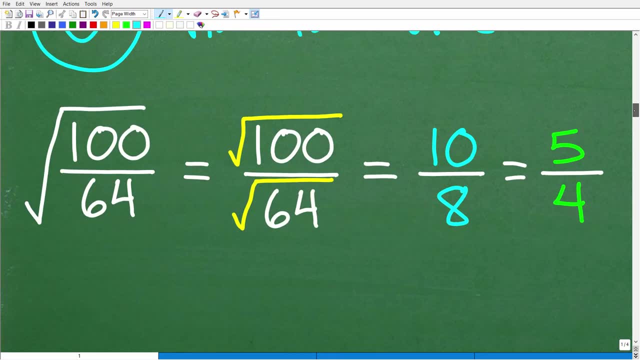 simplify this big thing over here into a much easier you know number, Okay, in other words, we're going to make the problem simpler, So let's go ahead and work on that right now. So the square root of 100 over 64, we need to understand there is a property of square root. 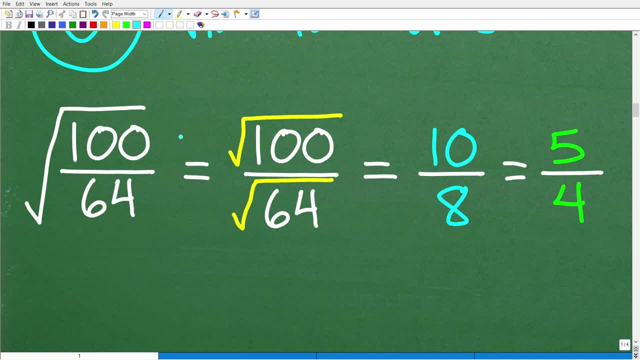 So the square root of a fraction we can break up as the individual square roots of the numerator and denominator. Okay, so you need to understand that. So the square root of 100 over 64 is equal to the square root of 100 over the square root of 64, the square root of 100 is 10, the square root. 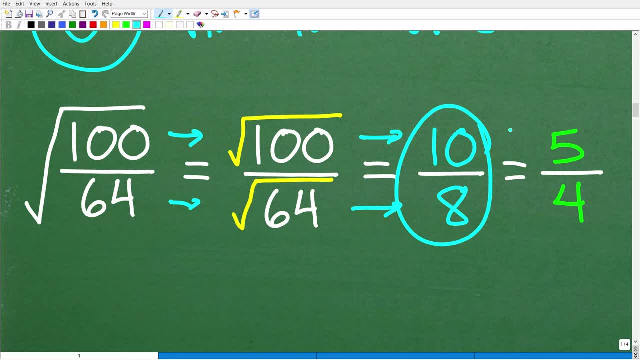 of 64 is eight, And so we have this fraction 10 over eight, which we can reduce down to five over four. right? two goes into 10, five and two goes into eight. all right, so instead of 100, or the square root of 100 over 64, let's replace all this stuff, right? 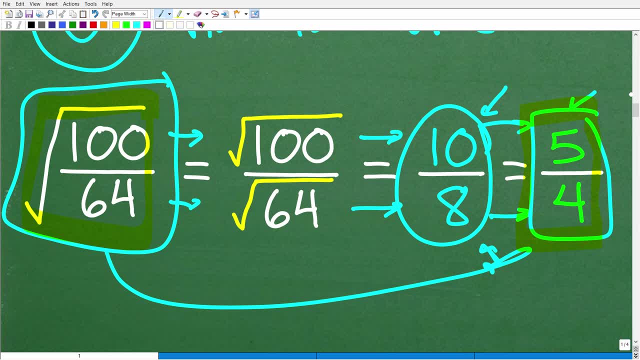 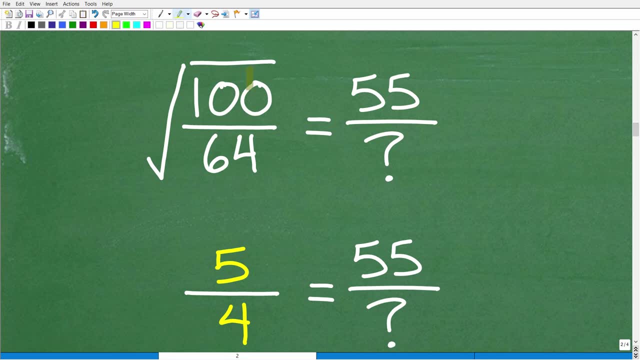 here with this lovely little fraction. right there, five over four, And now this becomes a lot easier to solve. Okay, so, instead of this problem, right here again, because we have this knowledge of working with square roots, we can just replace this entire numeric expression the square root. of 100 over 64 as five. So we're going to replace this entire expression, the square root of 100 over 64, as five over four. Okay, so, instead of this problem, right here again, because we have this knowledge of working with square roots, we can just replace this entire numeric expression, the square root. 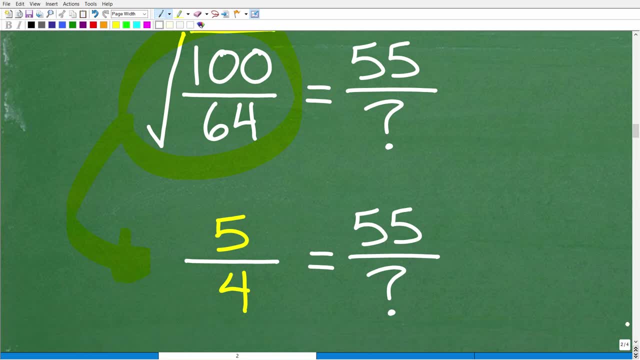 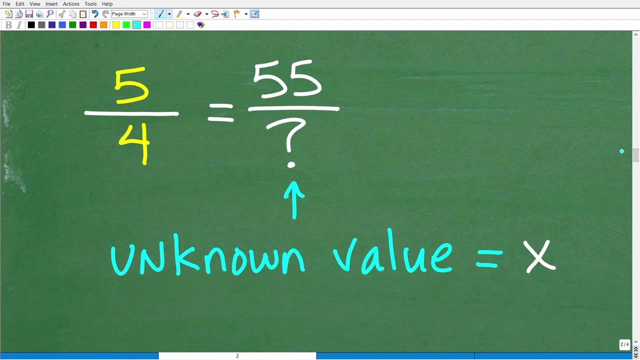 of 100 over 64 as five over four. Okay, so, instead of this problem- right here again, because we have this knowledge of working with square roots- we can just replace this entire numeric expression, the square root over four. This is a what, That's the union between the square root of 100 over 64 over 14.. Now next thing we're going to driving an IT strong macro system got to do a whole lot faster than we've done it, so you get a nice final result from it. So we want to do just fine for each and every qu? anciarety, because if you want a function that's not 라고, poke deep into youri. 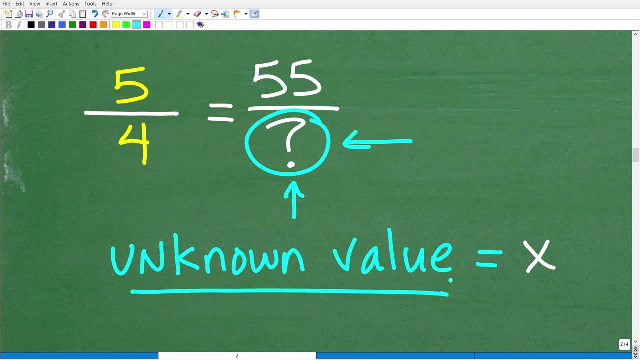 mark here is: we're looking for some unknown value, We're looking for the correct answer. Now, instead of a question mark, why don't we just replace this question mark with a symbol called a variable in mathematics or algebra, like x, right. So a variable again, symbols in. 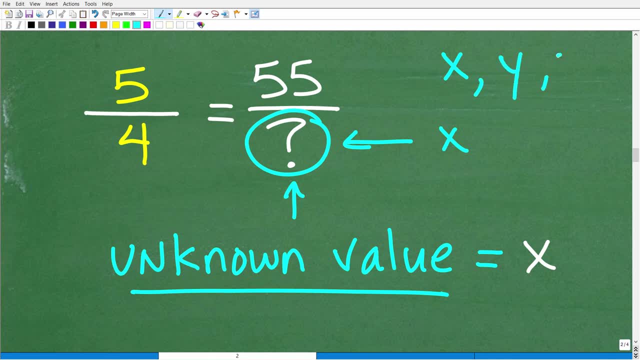 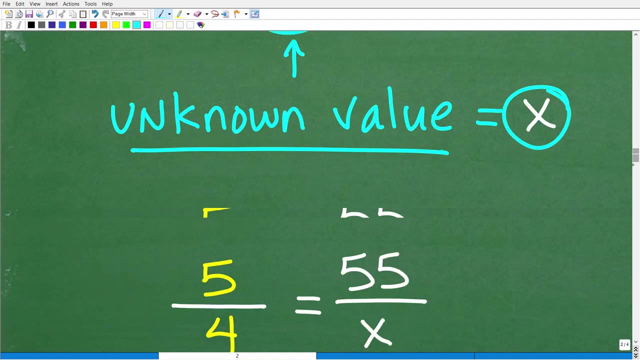 mathematics- and I'm talking about algebra here- like x, y, z, a, b, c, These things, these are variables. but what is a variable? A variable is just an unknown value. okay, So let's replace this question mark with an x. So now our problem is this: 5 over 4 is equal to 55 over x. 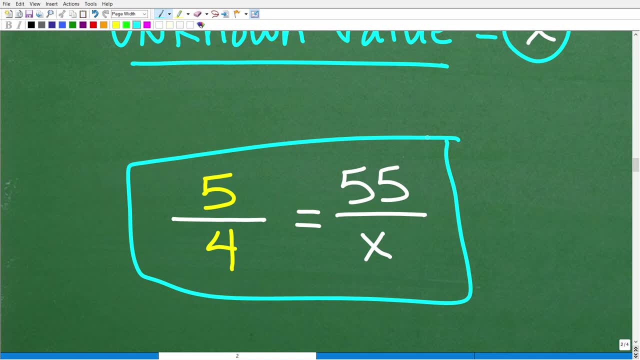 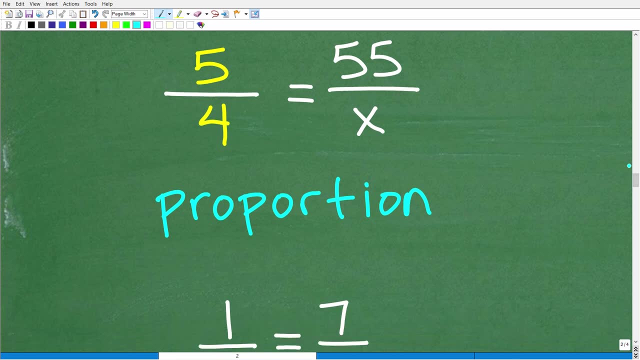 and now what we're talking about is a proportion problem. Okay, so what is a proportion? I'm going to go ahead and explain that right now. Okay, so here's our problem, and I keep calling this thing a proportion. So what is a proportion? Well, in uh. 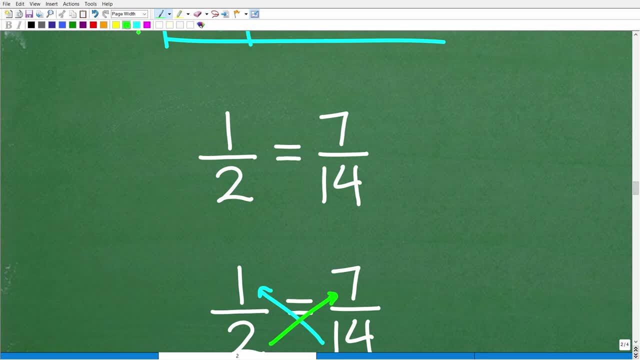 very simple terms, a proportion is nothing more than two equal fractions. So here's a fraction, let's say one half, and let's think of a fraction that is equal to the fraction one half. okay, Well, how about a fraction like 7 over 14,, or 3 over 6, or 5 over 10? It's any number of fractions. 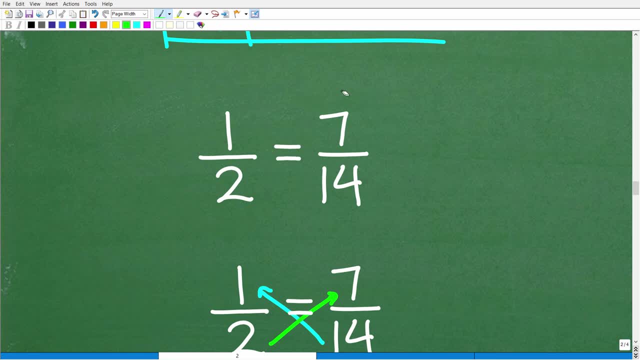 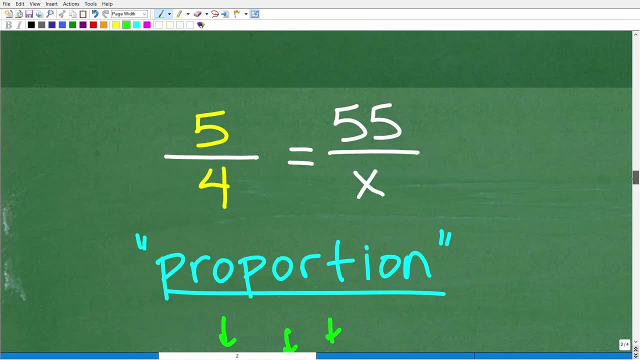 but these two fractions are equal and that is what a proportion is? This fraction is equal to this fraction, and that is our problem. Okay, let's take a look at our problem. We're saying this fraction is equal to this fraction. Well, in this fraction here, we just don't know the. 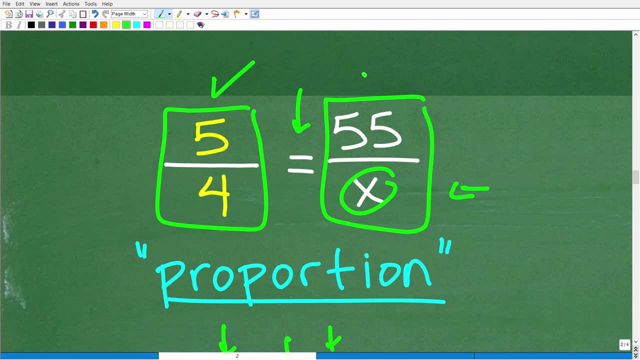 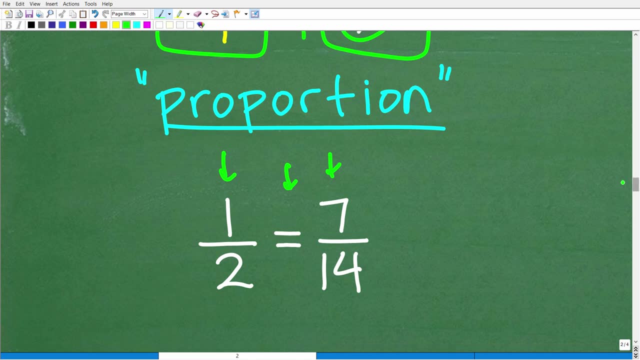 denominator, but it doesn't change the fact that we're saying that this fraction is equal to that fraction. Okay, now, what is the thing about proportions that we need to know? Well, when we have a valid proportion, an actual proportion, we have a great little property called the cross. 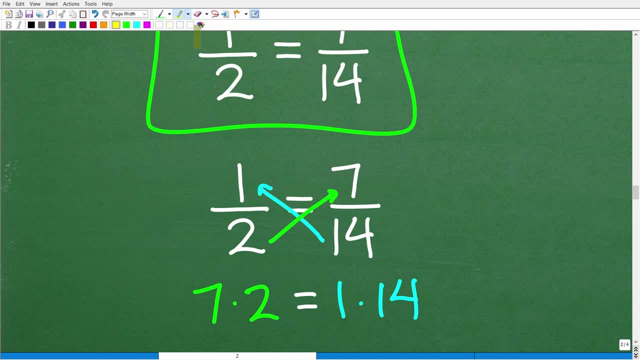 product, and what that means is, when we cross, multiply like this way, the cross products are equal, okay, So, in other words, here's a fraction and we're saying that this fraction is equal to this fraction. Okay, now what is the thing about proportions that we need to know? Well, in this. 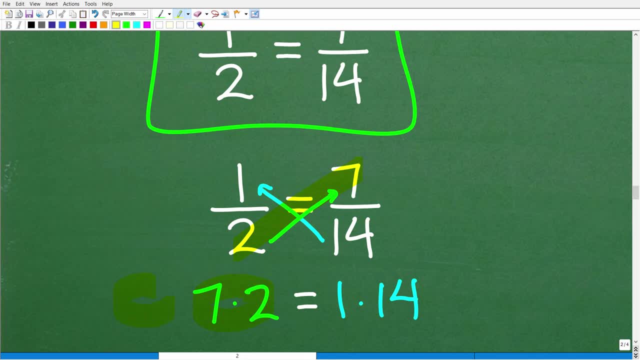 fraction here: 2 times 7 is what? Well, 2 times 7 is 14.. What's 1 times 14?? Well, that's 14.. So, when you have a proportion, we want to use the cross product. right, We're basically going to cross. 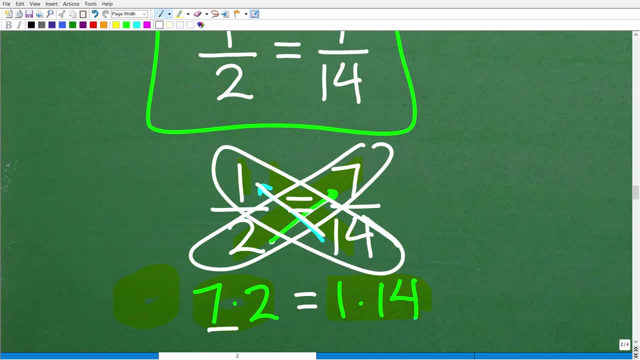 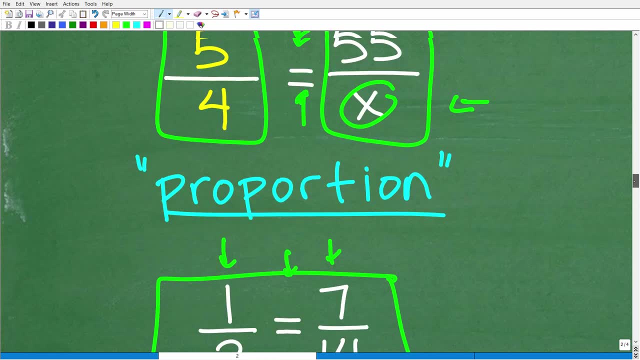 multiply, and the results of that cross multiplication are going to be equal. All right, so now that we understand the cross product, all we need to do is use some simple algebra to solve this proportion and solve the problem. So let's go ahead and take the next step, which, of course, 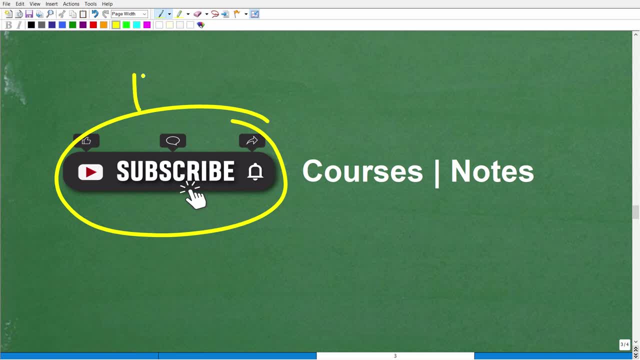 we're going to do, So let's go ahead and take the next step, which, of course, we're going to do. So let's quickly subscribe to my YouTube channel. I definitely need your help, and I'm not shy to ask for help because I have a goal. My goal is to reach as many people as I possibly can on YouTube. 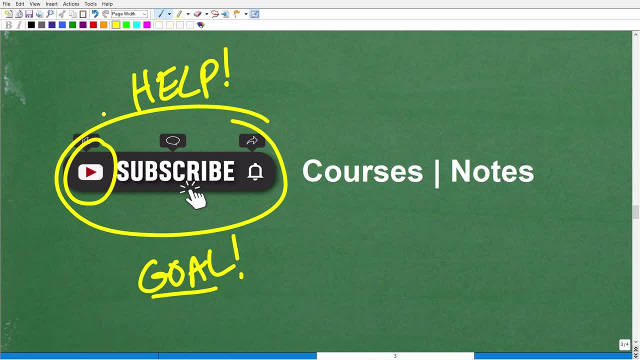 because I basically think of. every single person that watches my videos or subscribe to my channel is like my students and, as a math teacher, I'm happiest when I get as many people as possible in my classroom. okay, But I definitely need your help and the way you can support this channel. 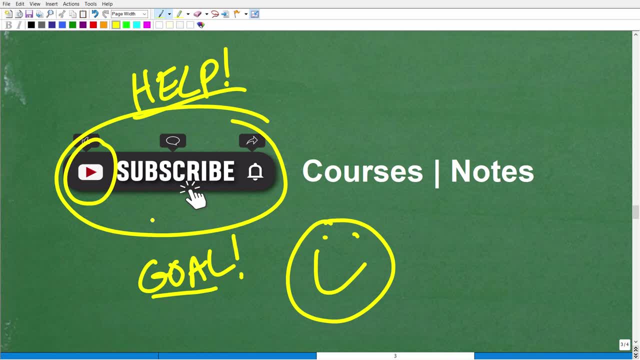 which is all about trying to make math clear and understandable and really try to encourage people to never give up in terms of learning mathematics. That's a big problem out there. A lot of people struggle in math and they think you know they start getting this thinking in their 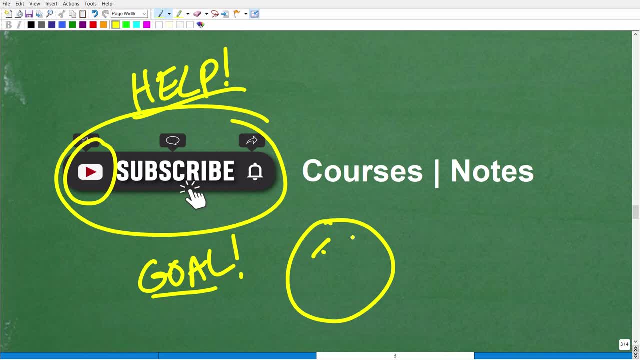 head. well, I'm just not smart enough to learn math, you know. you know, I'm just. it's the math's not my thing. I don't get it. Well, don't give up. okay, Math can be challenging, but what you need 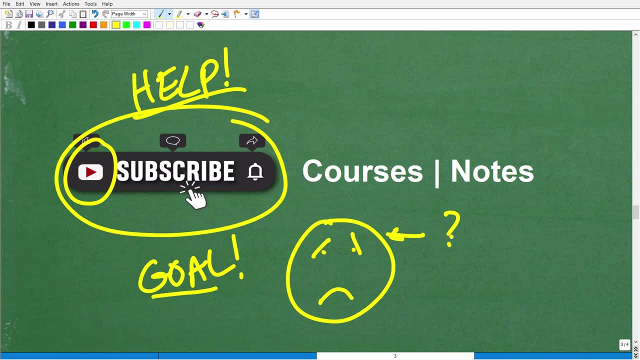 is encouragement. You need to kind of double down in, you know, in terms of your work ethic, but most importantly, you need great math instruction. and that brings me to my next point here. If you look at the links in the description of this video, you'll see basically. 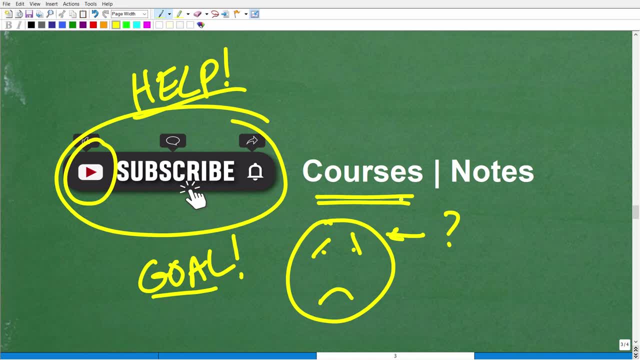 my full main or my most popular full math courses. all right, So this is where my best math instruction is going to be. They're very, very comprehensive math courses. so what we're talking about here- proportions- you can find you know these topics, or the topic of proportions basic. 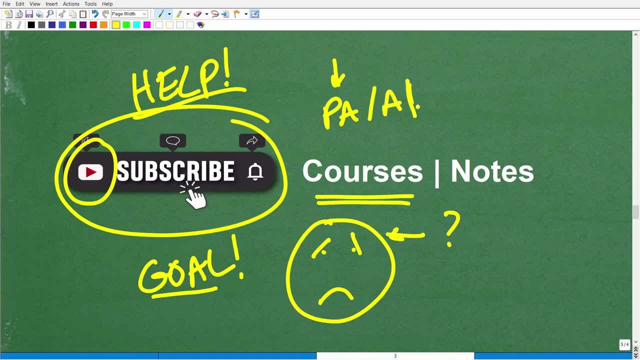 algebra in my pre-algebra course. I like my algebra course and if you just want to kind of get back to relearning mathematics, then check out my math skills, rebuild a course and if you just like to study from notes and whatnot, you like printable. 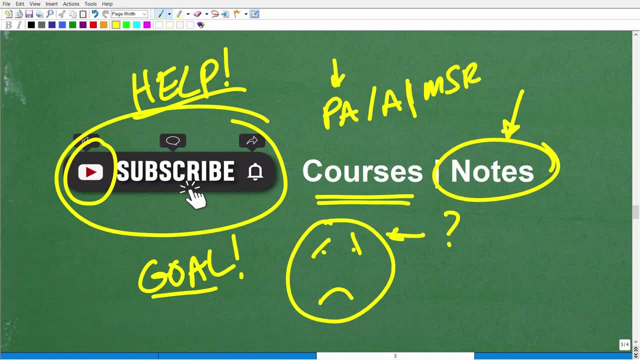 things. check out my link. I think it's called TC Math Shop. I actually should know that, but you'll see that link in the description and those are links to digital resources that you can download or print and pick up a set of math notes. All right, so don't forget to hit that notification. 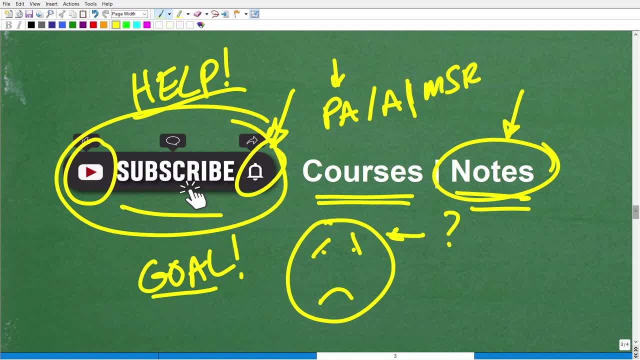 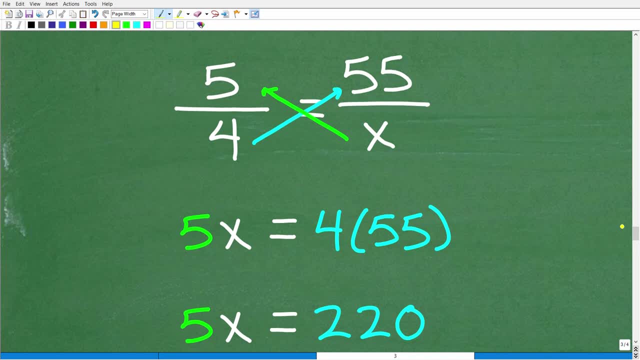 bell after you subscribe, so you can get my latest videos. and now let's go ahead and finish up this problem, because really there's not much to do. So what we're going to apply is the cross product. okay, We have a proportion. It's one fraction equal to another fraction, so we can. 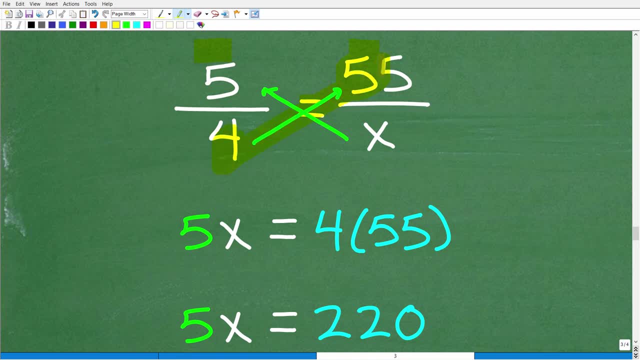 use the cross product. So 4 times 55,. we're going to multiply. this way is what We're going to write that right here. So 4 times 55 is equal to x times 5, all right. So this again is the application of. 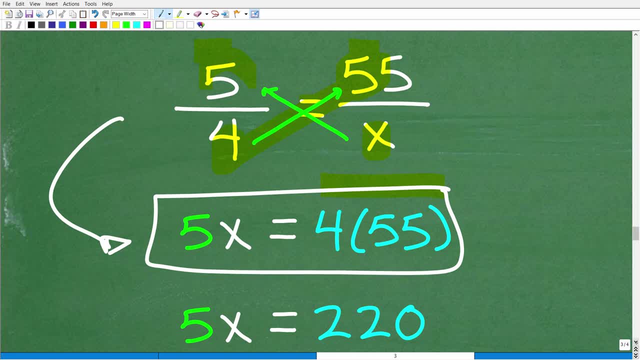 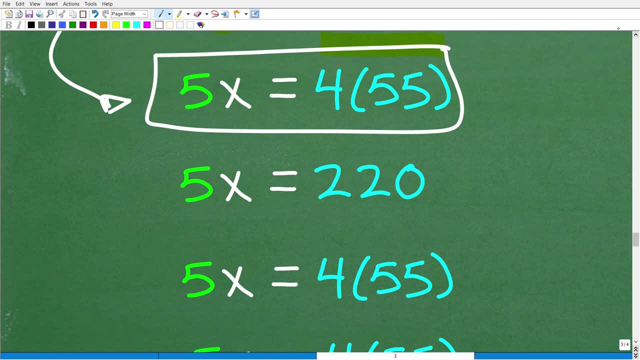 the cross product. Now we're going to solve this simple equation. Okay, now, right here, we have 4 times. oops, I kind of went a little bit too far. So we have 4 times 55. Now we could do the multiplication and get 220, but don't feel like you always have. 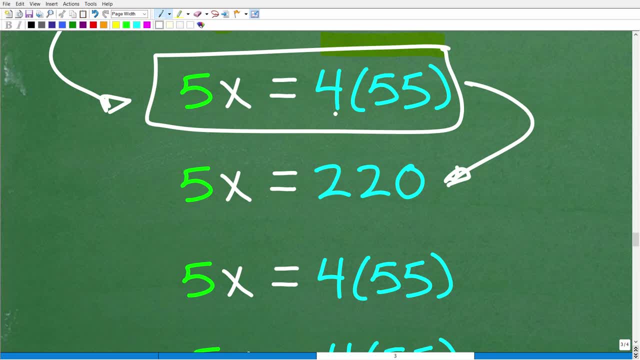 to multiply. okay. Now you might be saying: what are you talking about, Mr UT Math Man? Well, we have 4 times 55. Let's just think of the problem or the product as 4 times 55. I'm going to show. 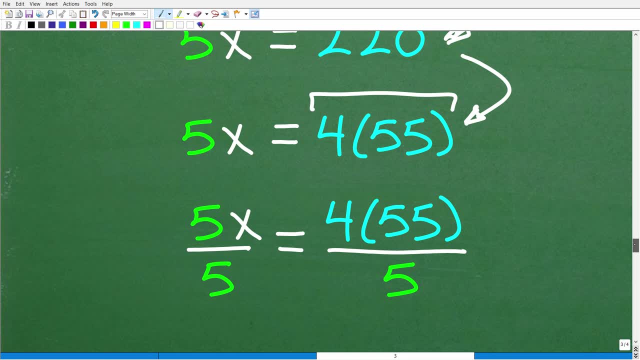 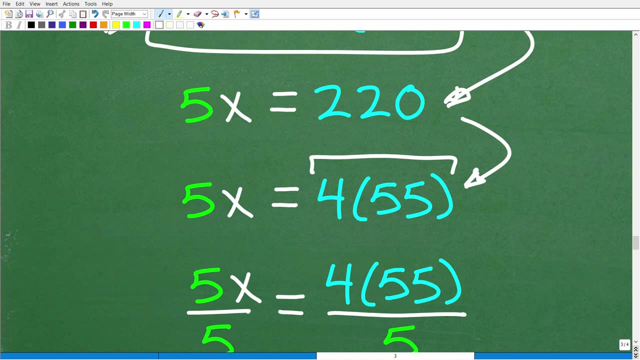 you a little bit of a reminder here: When you don't have a calculator, you can make your life a lot easier. Okay, so we know that we have this equation: 5x is equal to 220.. So to solve for x, I. 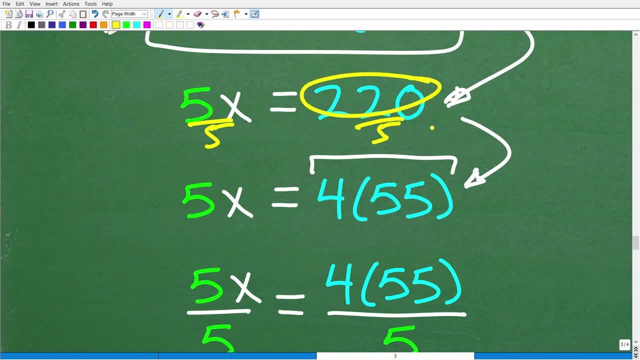 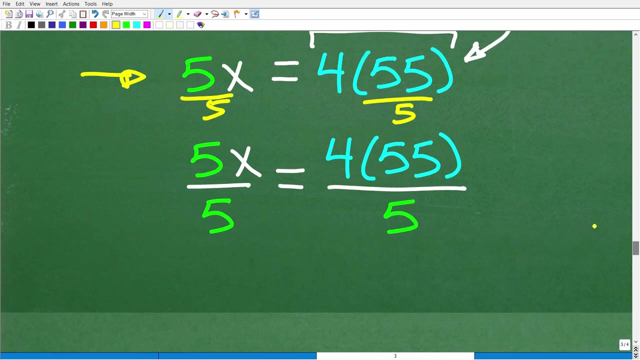 would have to divide both sides of the equation by 5. Again, 220 is the same thing as 4 times 55. But let's just solve the equation by dividing both sides of the equation by 5.. But here the numerator we're just going to leave as 4 times 55. Now, why would I do such a thing? Well it's. 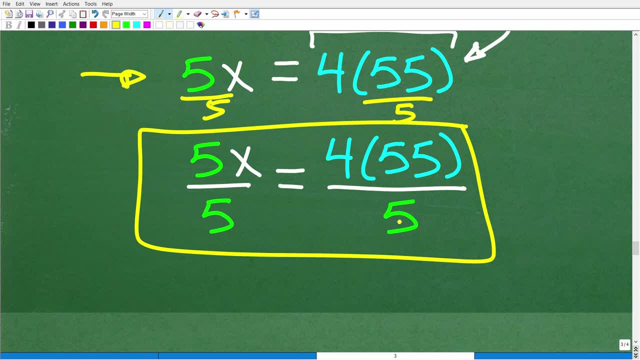 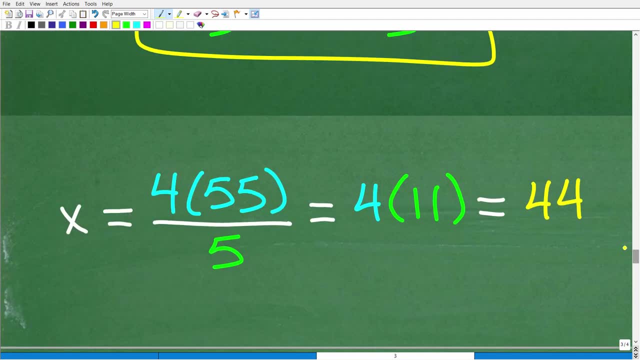 going to make our life easier. if we don't have a calculator because we have a 5 here, We have a 55 here, And to solve this problem, all we have to do is cross cancel. So in other words, we can. 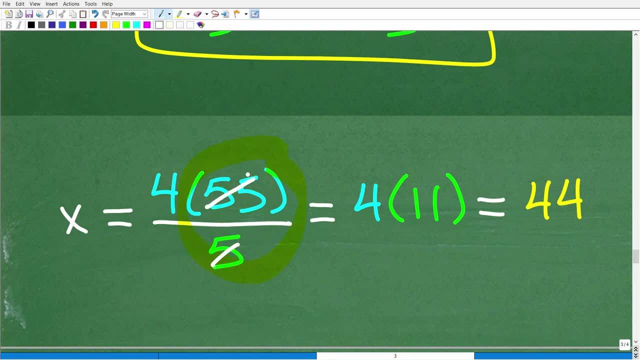 just look at this part of the problem: 5 goes into 55.. What 11, right? So if you have basic division skills you're like: oh yeah, 5 goes into 55, 11.. Well then, the answer is going to be 4 times 11,. 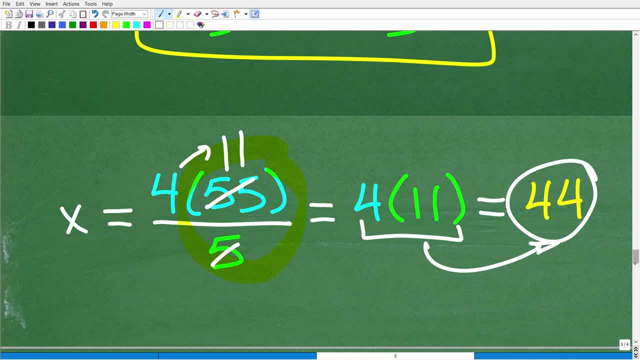 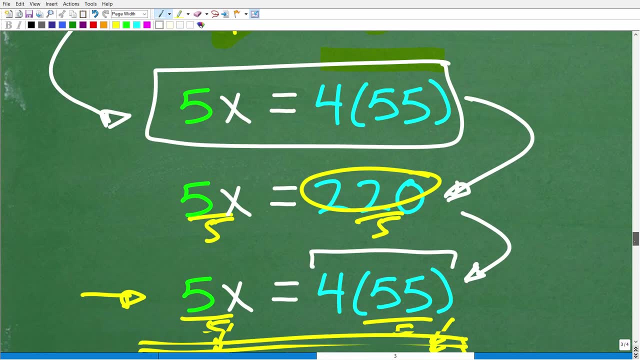 which of course is 44. So when you don't have a calculator, you want to kind of work as smart and as efficient as possible And oftentimes you're going to have to do a lot of work to get times. It's a good idea not to kind of do you know full-on multiplication until you know. 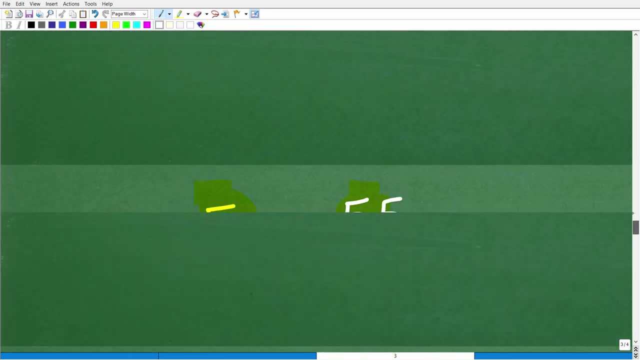 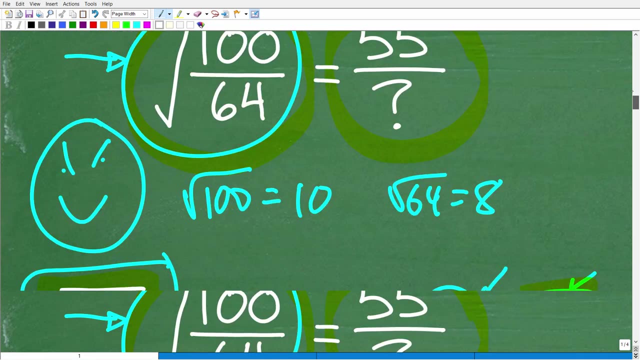 you absolutely have to. All right, So hopefully this was an interesting little problem in terms of square roots and proportions, But these are the basic math skills that you need to understand in order to be successful in things like algebra. But never feel bad if you don't understand. 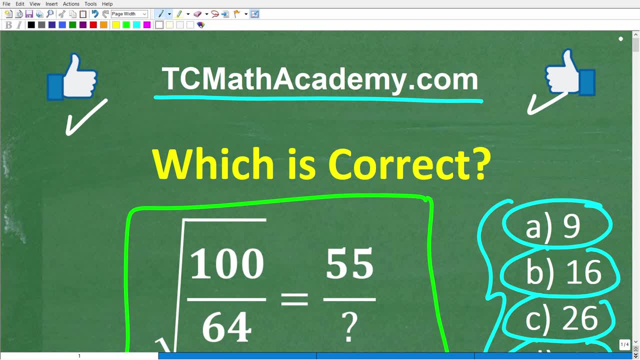 anything in mathematics. Use this as kind of a you know a list, if you will like. all right. I don't understand square roots as well Think or proportions, So it's like making yourself a little math shopping list, All right. 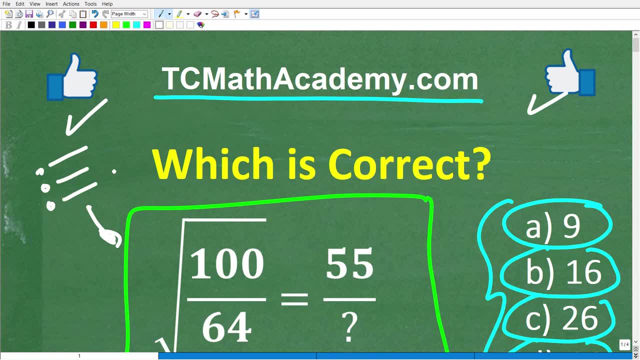 I got to pick up some proportion skills and some square root skills, etc. etc. And hopefully you got something out of this video And if that's the case, don't forget to like and subscribe. And, with that being said, I definitely wish you all the best in your math adventures. Thank you for your time and have a great day. 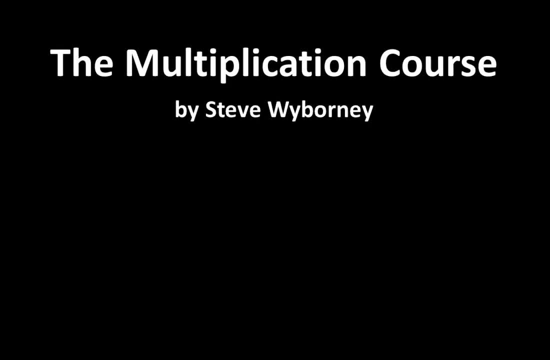 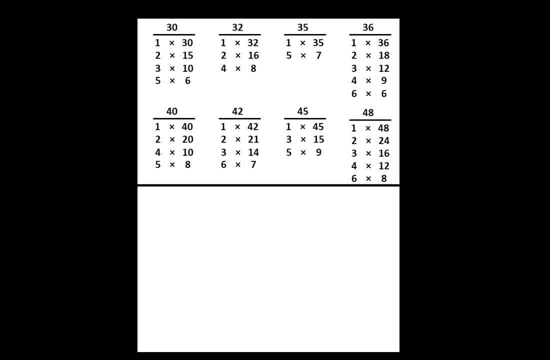 Welcome to the Multiplication Course. My name is Steve Wyborny and this is Finding Factor Pairs, Part 4.. In the last Finding Factor Pairs video, we completed the top half of the page. At the end of this video. your paper will look like this Throughout this video, if you need. 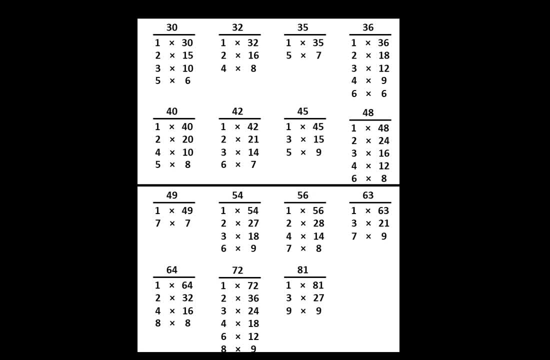 more time at any point. simply pause the video and take as much time as you like To prepare the paper. write these numbers and underline them too. Write 49 and underline it. Then write 54 and underline it. Now write 56,, 63,, 64,, 72, and 81,, which is the last one. Again, if you need, 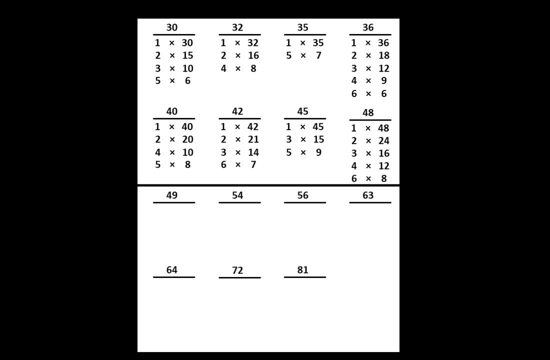 more time, simply pause the video. Let's begin with the number 49.. On your paper write that we can think of 49 as 1 times 49.. Or 7 times 7.. Those are all the factor pairs of 49.. 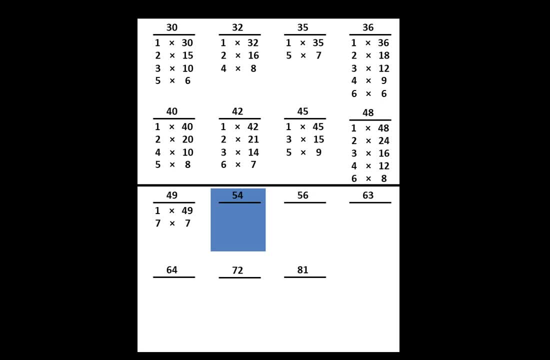 Let's move to the number 54. On your paper, write that we can think of 54 as 1 times 54. Or 2 times 27. Or 3 times 18. Or 6 times 9..